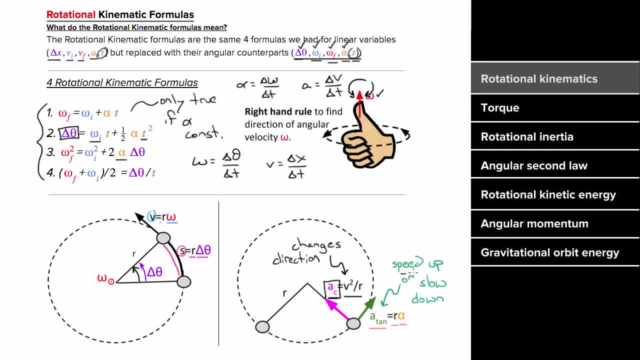 because it's changing directions, But only if it's speeding up or slowing down will it have tangential acceleration and angular acceleration. So what's an example problem involving the angular motion variables? look like, Let's say, an object is rotating in a circle at a constant rate. 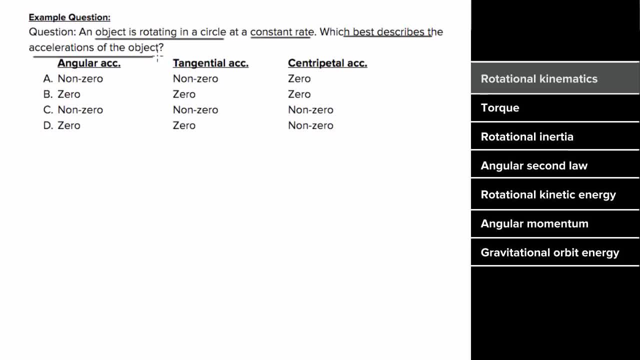 Which would best describe the three different types of accelerations of the object? Well, if an object's moving in a circle at all, there has to be centripetal acceleration, So that's got to be non-zero. And if it's rotating at a constant rate, 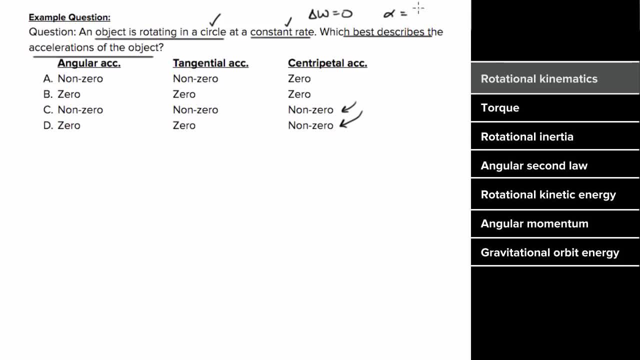 there's no change in omega, And that means the angular acceleration is going to be zero. If the angular acceleration is zero, the tangential acceleration would also be zero. Only when the object is speeding up or slowing down do you have angular acceleration and tangential acceleration. 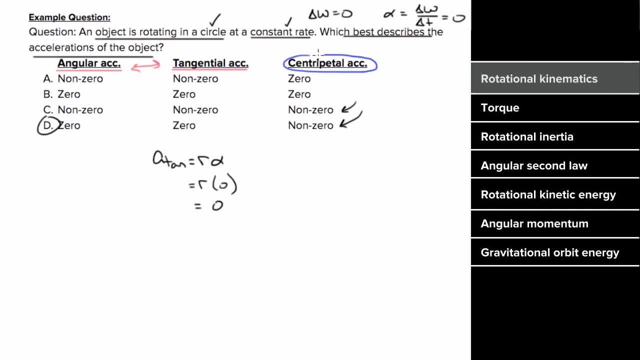 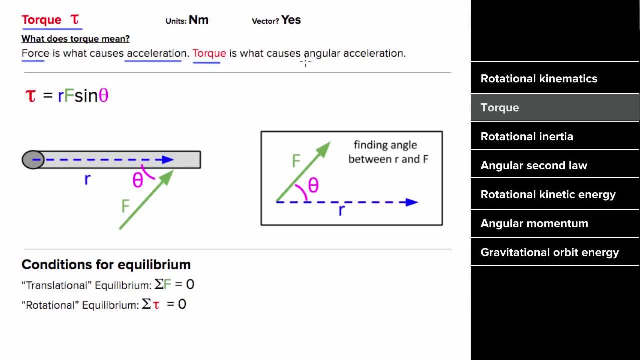 These change the speed, and centripetal acceleration changes the direction. What does torque mean? Just like force is what causes acceleration, torque is what causes angular acceleration. So in order for an object to speed up or slow down in its angular motion, 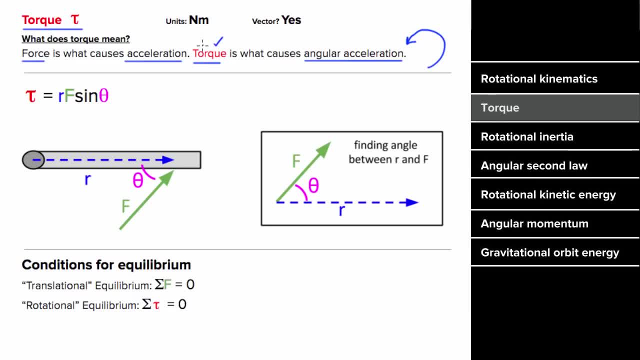 there's got to be a net torque on the object. What causes a torque? Forces cause torque. So in order to have a torque you have to have a force. But the same force could exert a different torque depending on where that force is exerted. 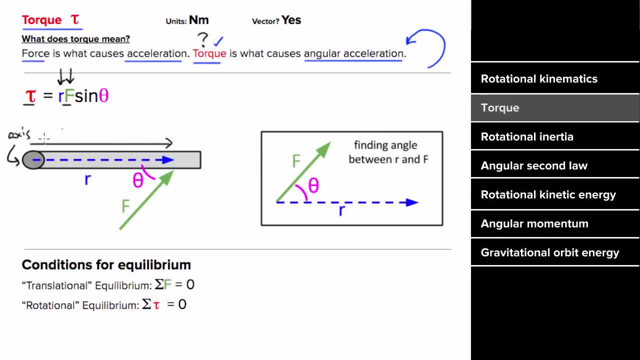 If the force is exerted far from the axis of rotation, you'll get more torque for that given amount of force compared to forces that are exerted near the axis of rotation. This R represents how far that force is applied from the axis, And to maximize that force you would actually want to point it perpendicular to this R. 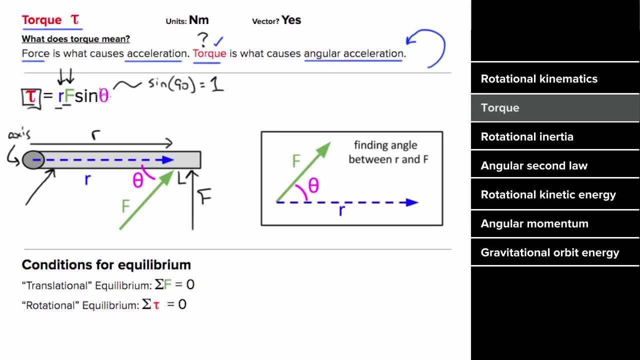 since sine of 90 degrees is equal to 1.. So, in other words, to maximize the amount of torque you get, exert the force as far away as possible from the axis and exert that force perpendicular to the line from the axis to that force. 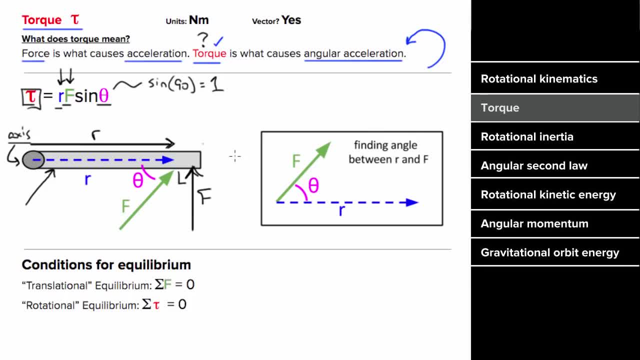 You might get many angles in a problem, but this angle here is always the angle between the R and the F, And just like an object is in translational equilibrium if the net force is zero, we say that an object is in rotational equilibrium if the net torque is zero. 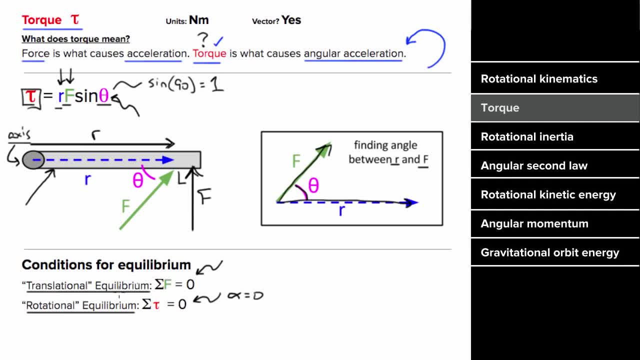 This would cause the angular acceleration to be zero, just like translational equilibrium causes the acceleration to be zero. Torque is a vector, so it has a direction. Typically, it's easiest to think of the direction as just being counterclockwise or clockwise. 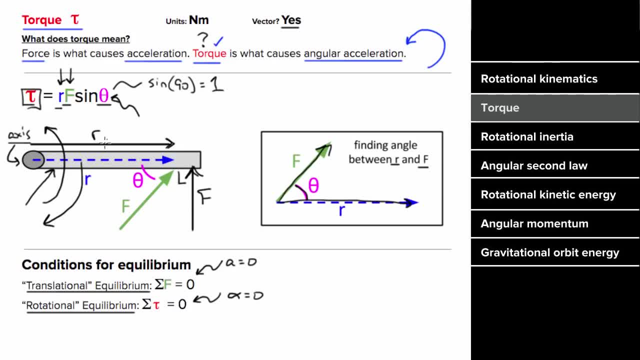 based on which way that force would cause the object to rotate. And since torque is R times F, the units are going to be meters times Newton or Newton meters. So what's an example problem involving torque? look like, Let's say, you had this rod with this axis here. 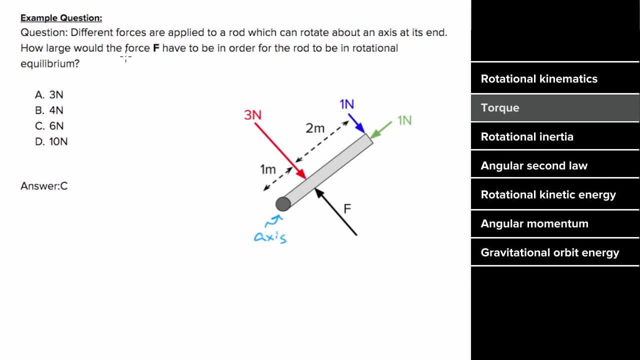 and there were forces applied as shown. We want to know how large would the force F have to be in order for this rod to be in rotational equilibrium? So remember, rotational equilibrium means that the net torque is equal to zero, In other words, all the torque that's pointing clockwise. 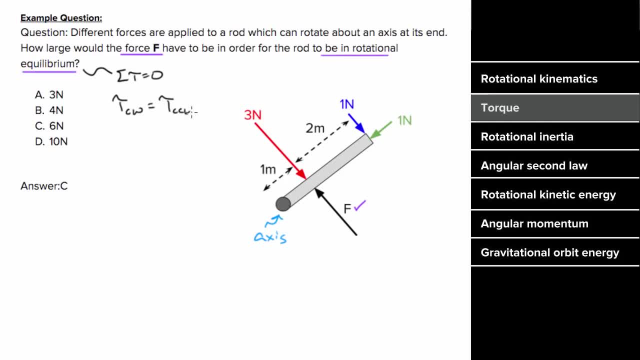 would have to equal all the torque that points counterclockwise in order for the system to be balanced. The three-Newton force and the one-Newton force is trying to rotate this system clockwise and the unknown force F is trying to rotate the system counterclockwise. 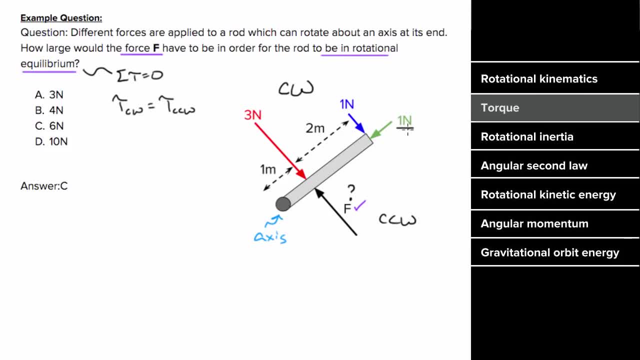 This green one-Newton force isn't actually exerting any torque, Even though the R value is not zero. the angle between the force and the R value is going to be 180 degrees and the sine of 180 degrees is zero, which makes sense since this force isn't actually causing this rod. 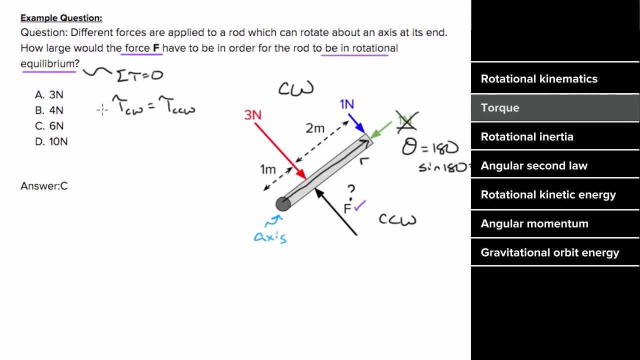 to rotate clockwise or counterclockwise, So the torque in the clockwise direction would be one meter times three Newtons. To find the torque from the three-Newton force Plus you wouldn't use two meters for the R of the one-Newton force. 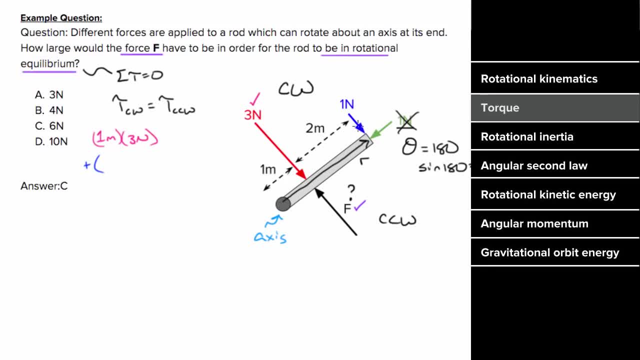 You have to find the R from the axis, which is going to be three meters times one-Newton force, which gives a total clockwise torque of six-Newton meters. And we could write the torque applied by the unknown force, F, as one meter times F. 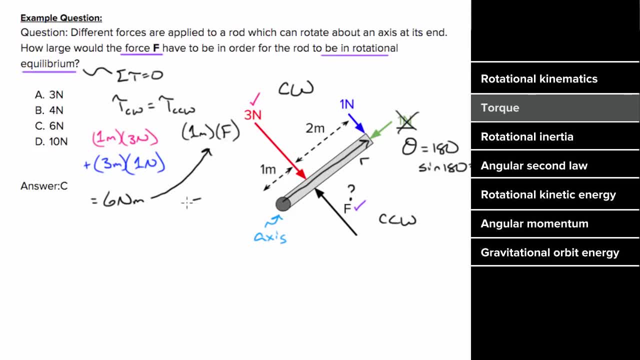 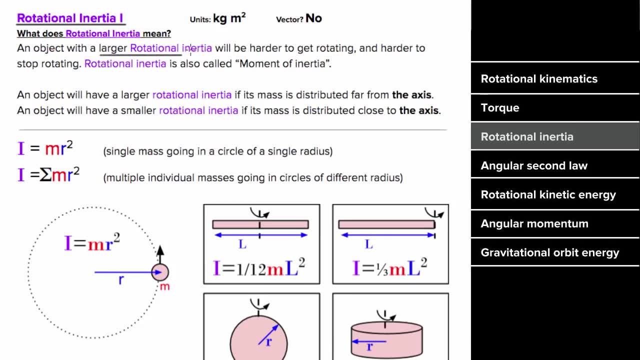 So in order for six-Newton meters to equal one times F, the force F just has to equal six Newtons. What's rotational inertia mean? Well, an object with a large rotational inertia will be hard to get rotating and harder to stop rotating. 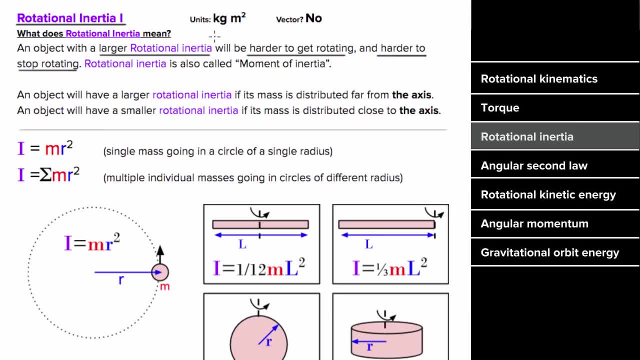 Basically, the rotational inertia tells you how much an object will resist angular acceleration, Just like regular inertia tells you how much an object will resist regular acceleration, And this rotational inertia is often referred to as the moment of inertia. How do you make the rotational inertia large? 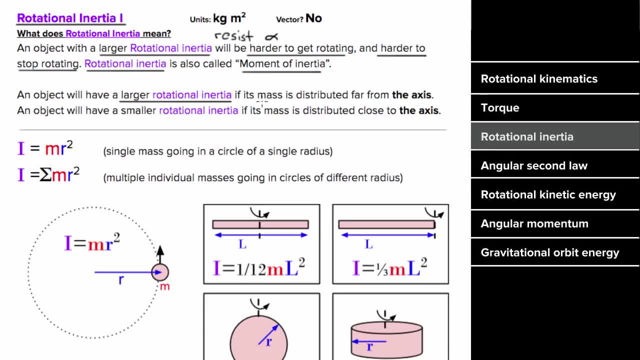 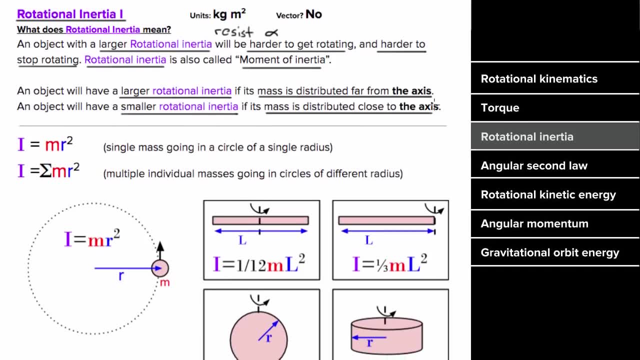 Well, you can increase the rotational inertia if you place the mass far from the axis of rotation. And you can make the rotational inertia smaller if you place the mass closer to the axis of rotation. In other words, if you could push the mass closer to the axis of rotation. 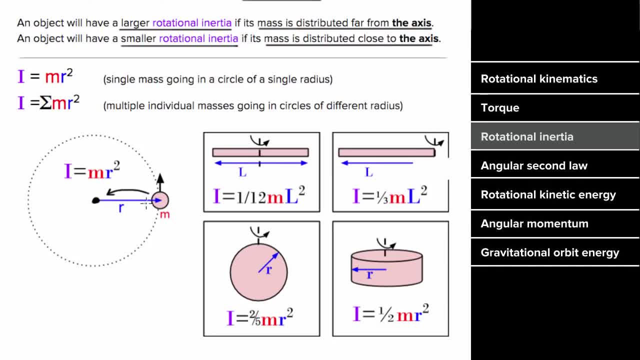 which is the point about which the object rotates. you could make the moment of inertia smaller and smaller. To find the moment of inertia, or rotational inertia, of an object whose entire mass rotates at the same radius r, you can just use the formula: 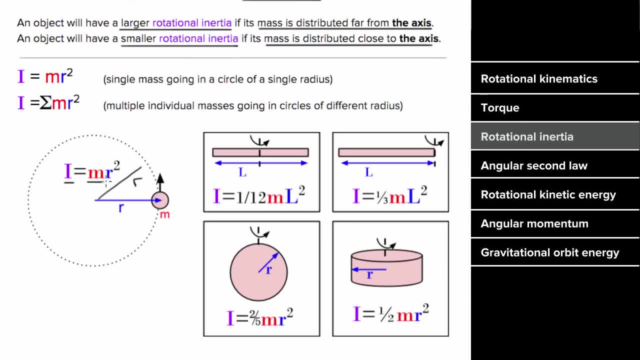 I equals the mass, that's rotating times, how far it's rotating from the axis squared. This formula's not given, You have to memorize it. I equals m r squared, And if you had many masses rotating at different r's you could just add up all the contributions. 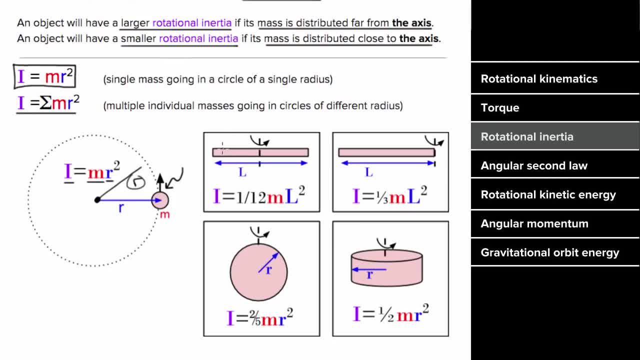 from each single mass. Now if you have a continuous object whose mass is not all at the same radius from the axis, the formulas are a little more complicated. For a rod rotating about its center, the moment of inertia would be one twelfth. 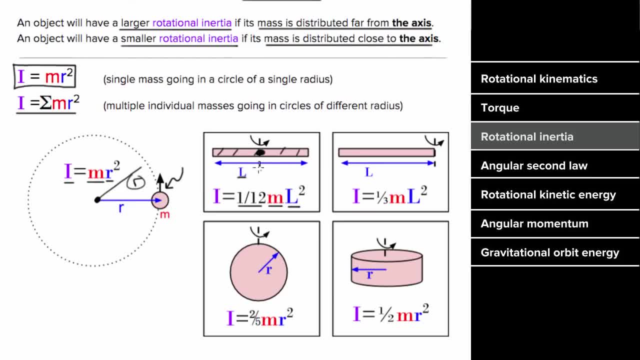 the mass of the rod times the entire length of the rod squared. For a rod rotating about one end, the moment of inertia's gonna be larger, since more mass is distributed farther from the axis, And this formula's one third the mass of the rod. 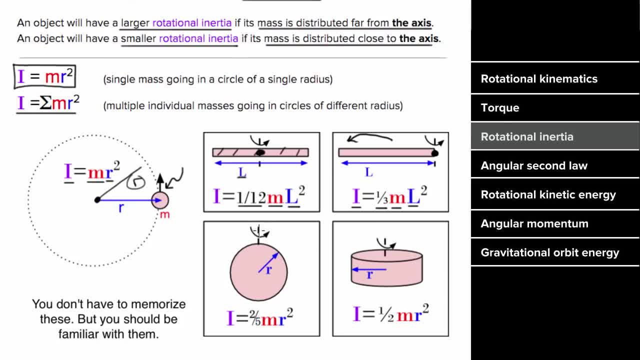 times the entire length of the rod squared. The rotational inertia of a sphere rotating about an axis through its center would be two fifths the mass of the sphere, times the radius of the sphere squared, And the rotational inertia of a cylinder or a disk rotating about an axis through its center. 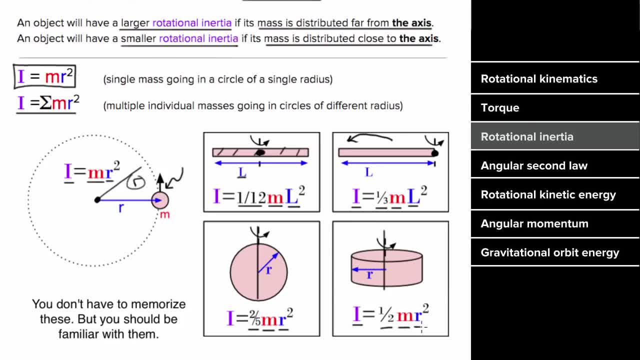 would be one half the mass of the disk times the radius of that disk squared. Another example that comes up a lot, that you wouldn't be given the formula for is a hoop, That is to say where all the mass is distributed around a center point with a hollow center. 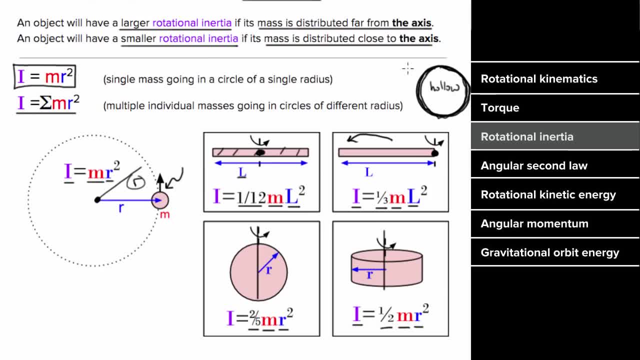 Since all the mass is at the same radius r, the formula for the rotational inertia of a hoop is just the same as the formula for the rotational inertia of a single mass rotating at radius r. The fact that the mass is distributed in a circle doesn't actually matter, since the mass 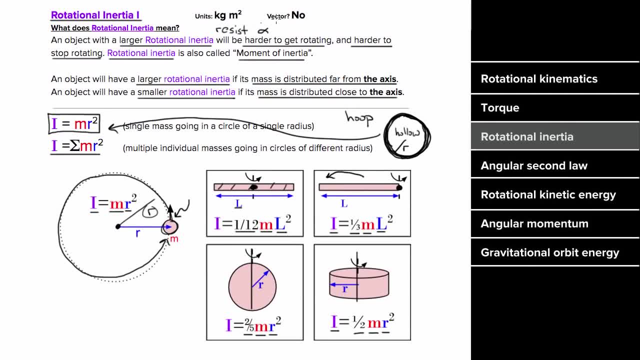 still stayed at the same radius r away. Rotational inertia is not a vector, so it's always positive or zero And the units, since it's m? r squared, would be kilograms times meters squared. So what's an example problem involving rotational inertia? look like. 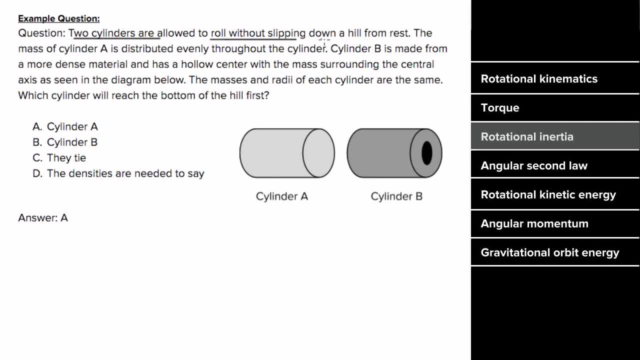 Let's say two cylinders are allowed to roll without slipping from rest down a hill. The mass of cylinder A is distributed evenly throughout the entire cylinder. Cylinder B is made from a more dense material and it has a hollow center with the mass distributed around that hollow center. 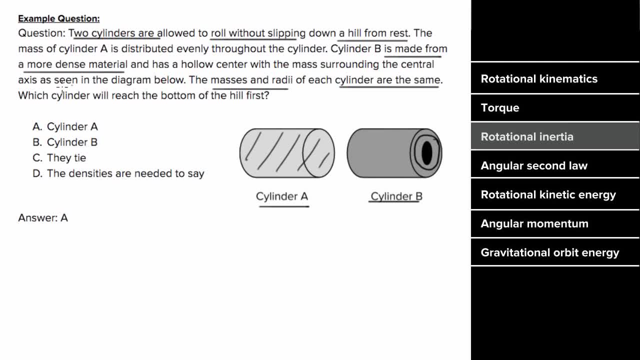 If the masses and radii of the cylinders are the same, which cylinder would reach the bottom of the hill first? To figure out which cylinder gets to the bottom of the hill first, we have to ask which one would roll more readily: The cylinder with the least moment of inertia? 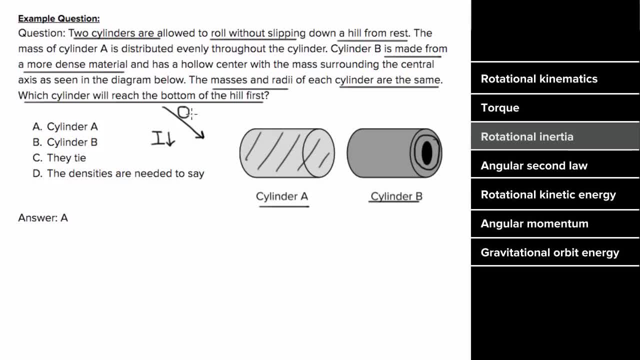 is going to be easier to rotate. That means it would roll more readily and get to the bottom of the hill faster. Whenever the mass is distributed farther away from the axis, the object is going to have a larger moment of inertia. So since the mass of cylinder B overall, 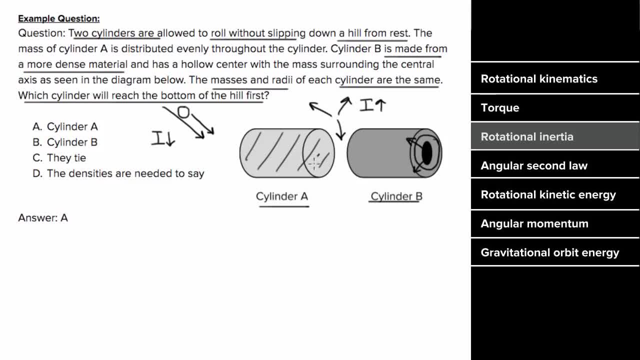 is farther away from the axis compared to cylinder A. cylinder B has a larger moment of inertia. That means it's harder to rotate, it will take longer to get down the hill and cylinder A is going to win. What's the angular version of Newton's second law? 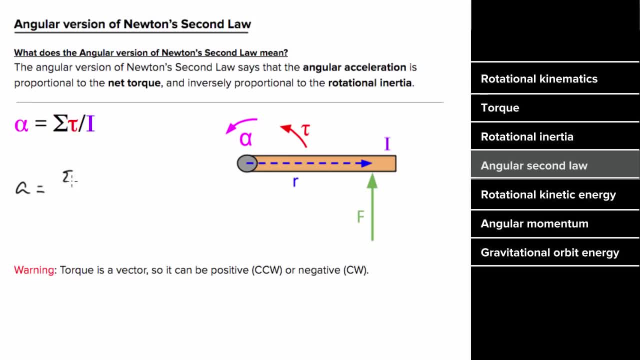 Well, Newton's second law says that the acceleration is equal to the net force divided by the mass, And the angular version of Newton's second law says that the angular acceleration is equal to the net torque divided by the rotational inertia. M tells you how much an object resists acceleration. 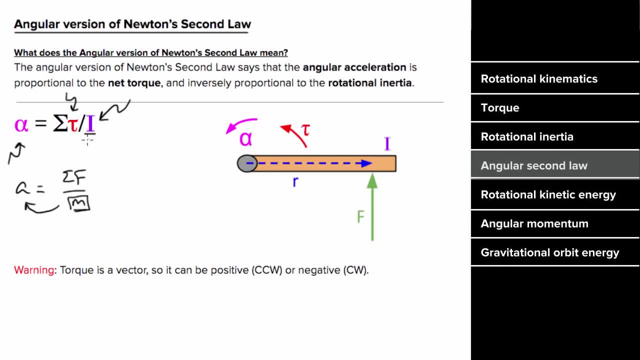 And the moment of inertia, or rotational inertia, tells you how much an object resists angular acceleration. So just like when you add up force vectors, you have to be careful with positive and negative signs, the same holds true with the torque vectors. 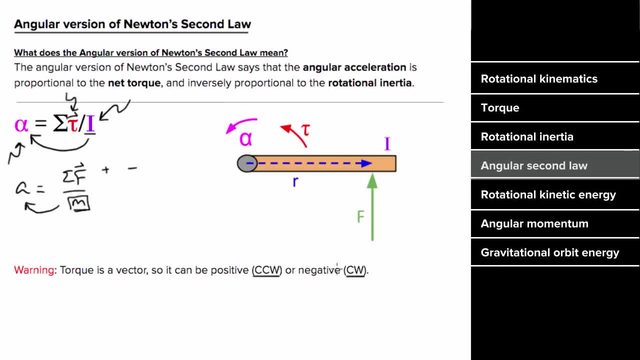 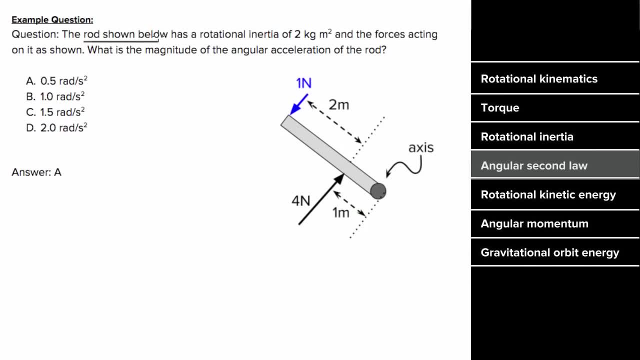 You've got to treat either counterclockwise or clockwise as positive and then be consistent with it. So what's an example problem involving the angular version of Newton's second law? look like, Let's say, the rod shown below has a rotational inertia of 2 kilogram meters squared. 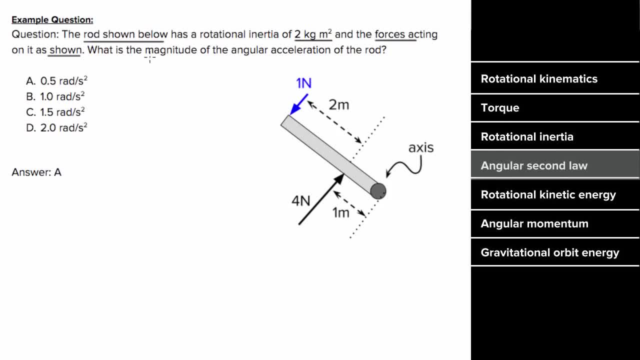 and has the forces acting on it as shown. We want to know what the magnitude of the angular acceleration is of the rod, So we use Newton's second law in angular form, which says that the angular acceleration is the net torque divided by the rotational inertia. 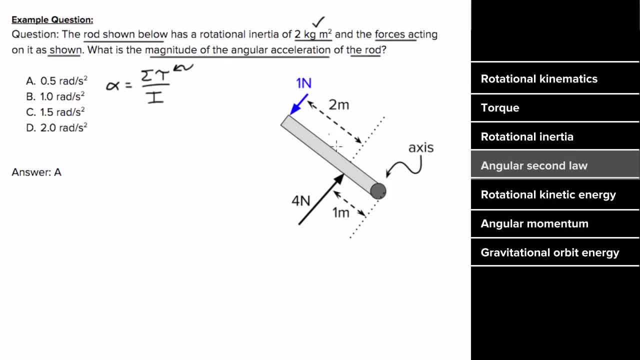 We've got the rotational inertia, we just need the net torque. So we have to figure out the total torque from all these forces. The torque from the 1 Newton force would be r, which is going to be 3 meters from the axis to that force, 1 Newton. 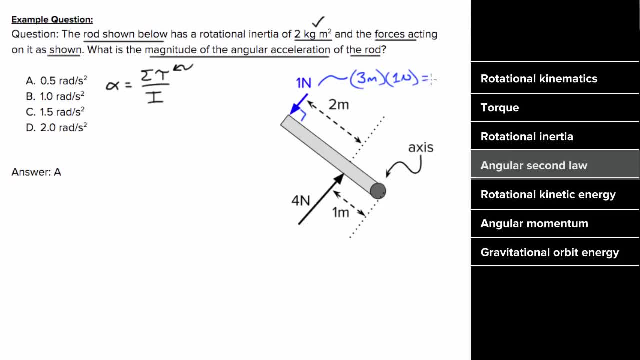 And since it's applied, perpendicular, the sine of 90 is going to be 1.. So the torque from the 1 Newton force would be 3 Newton meters and the torque from the 4 Newton force would be 1 meter. since it's applied, 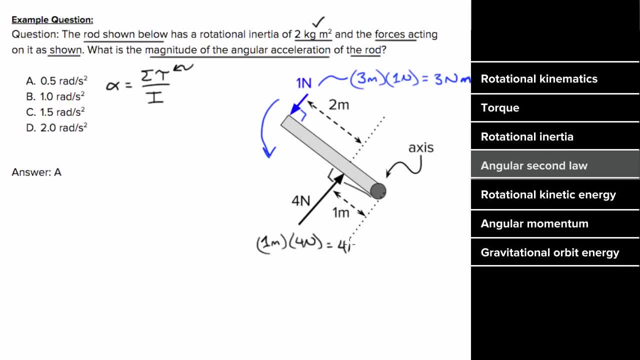 1 meter from the axis times 4 Newtons And we get 4 Newton meters in the clockwise direction. That means the total net torque when you have 4 Newton meters in the clockwise direction and 3 Newton meters in the counterclockwise direction. 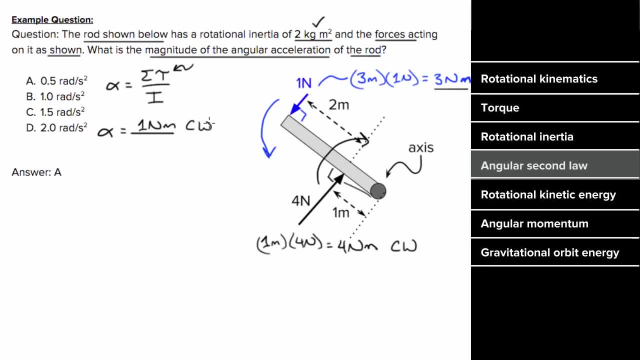 would just be 1 Newton meter in the clockwise direction, since 4 is 1 unit bigger than 3.. And now we divide by the rotational inertia, which was 2, which gives us an angular acceleration of 1 half and 1.5. 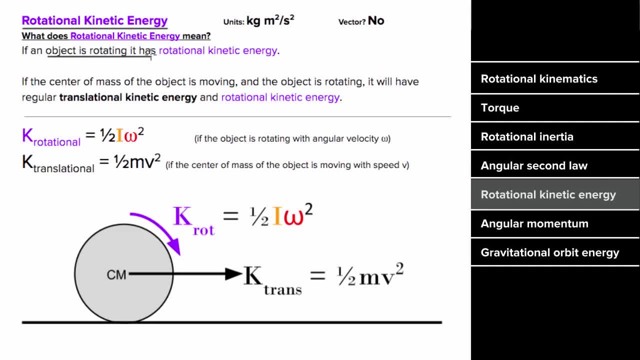 What's rotational kinetic energy mean? Well, if an object is rotating or spinning, we say it has rotational kinetic energy. If the center of mass of an object is moving and the object is rotating, we typically say that object has translational kinetic energy. 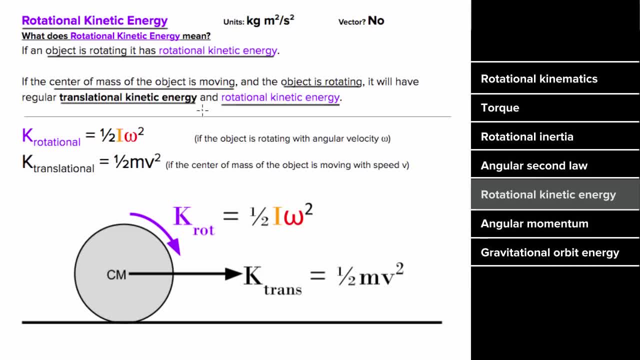 and rotational kinetic energy. They're both kinetic energies. this is just a convenient way to delineate between two types of kinetic energy and a particularly convenient way to find the total kinetic energy for something that's moving and rotating 1 half times the moment of inertia. 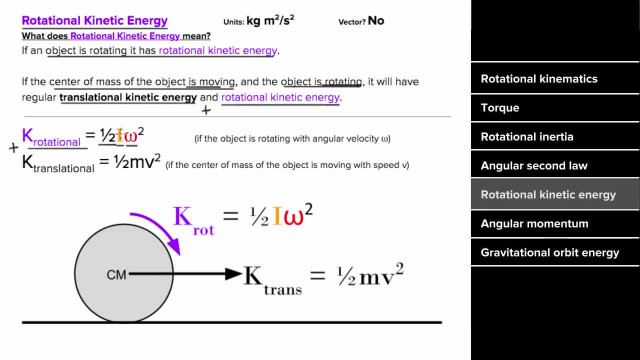 or the rotational inertia times the angular speed squared, which makes sense because the formula for regular kinetic energy is 1 half times the regular inertia, the mass times the regular speed squared. So again, if an object is rotating, it's got rotational kinetic energy. 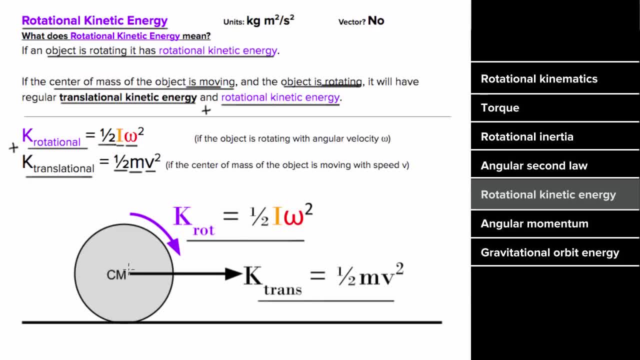 If the center of mass of an object is moving, it's got regular translational kinetic energy. And if the center of mass is moving and the object is rotating, then we say that object has both rotational energy and translational energy. It's not a vector. 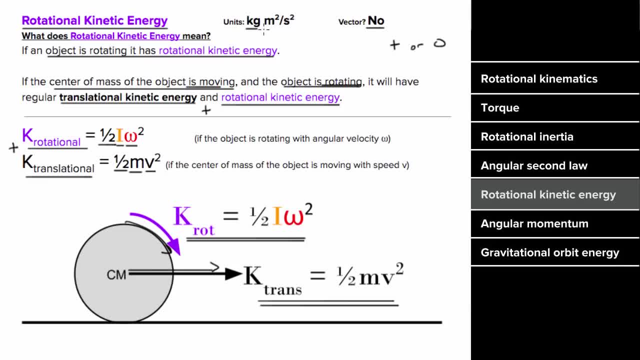 It is always positive or zero And the units can be written as kilogram meter squared per second squared. but it's an energy, so we know that just has to equal joules. So what's an example problem involving rotational kinetic energy? look like. 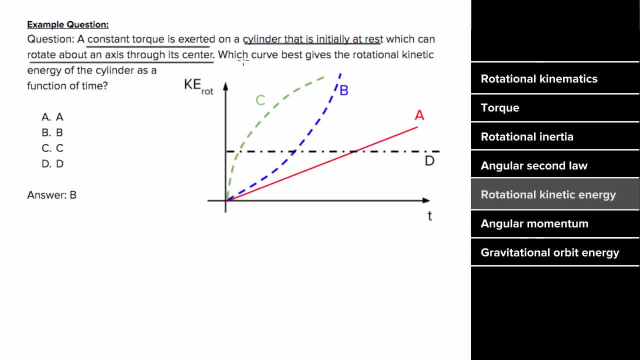 Let's say a constant torque is exerted on a cylinder that's initially at rest and can rotate about an axis through its center. Which of these curves would best give the rotational kinetic energy of the cylinder? as a function of time, It will cause a constant angular acceleration. 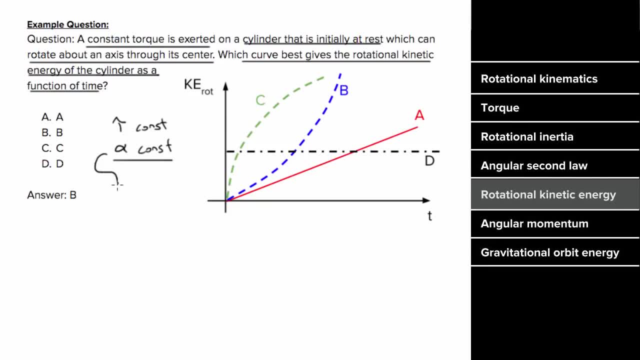 And if the angular acceleration is constant, we can use the kinematic formulas to figure out the final velocity of this object. The final angular velocity if it started at rest would just be alpha times t. That means the rotational kinetic energy of this object could be written as: 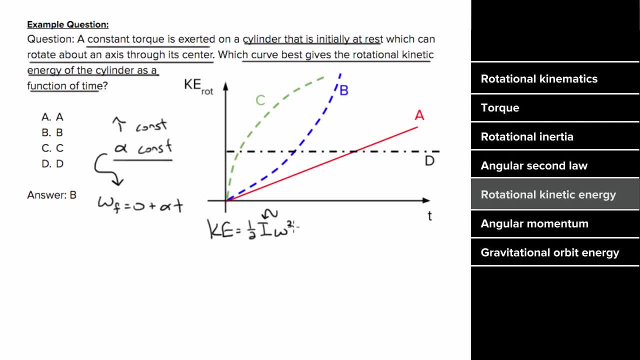 one half the moment of inertia, which is a constant times omega squared, which in this case would be one half i times alpha t squared. So, since the function for kinetic energy would be the time squared, if you graphed kinetic energy as a function of time, 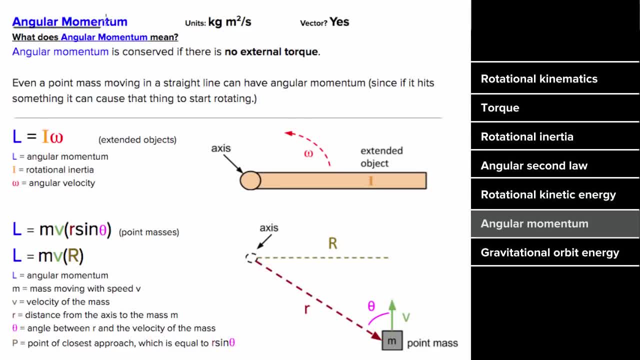 it would look like a parabola, so the correct answer would be b. What's angular momentum? Well, the reason we care about angular momentum is that it will be conserved for a system if there's no external torque on that system, And just like regular momentum, 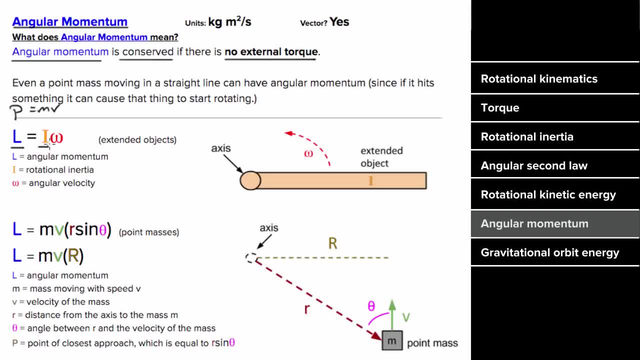 is mass times velocity. angular momentum will be the rotational inertia times the angular velocity, And this is a convenient formula to find the angular momentum of an object whose mass is distributed at different points away from the axis of rotation. The strange thing about angular momentum. 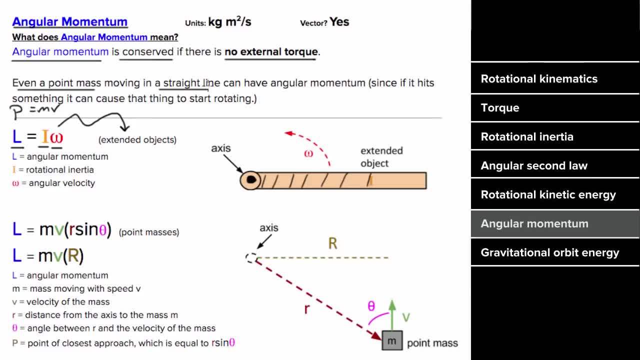 is that even a point mass moving in a straight line can have angular momentum. To find the angular momentum of a point mass moving in a straight line, take the mass of the object times the velocity of that object, and either multiply by how far that object is from the axis. 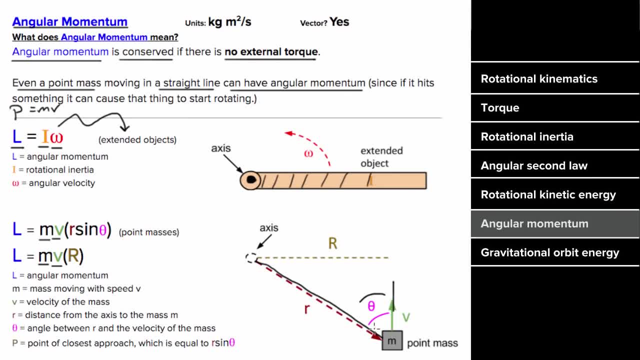 times sine of the angle between the velocity vector and that r. or the easier way to do it is to just multiply by the distance of closest approach, which is how close that mass will ever get to or ever has been from the axis, In other words, to determine the angular momentum. 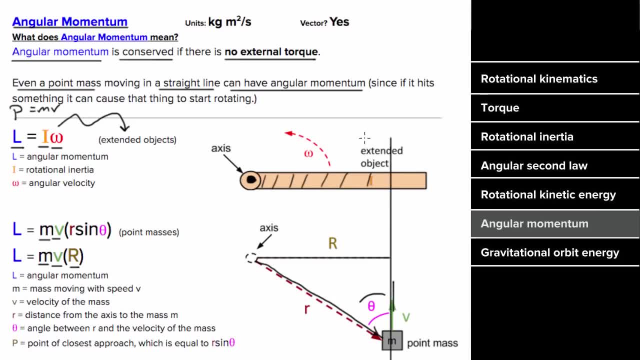 of this mass moving in a straight line, draw a straight line along its trajectory and ask: how close has it gotten, or ever will get to the axis? That's the capital R I'm talking about and if you take that, times the mass, times velocity, you'll get the 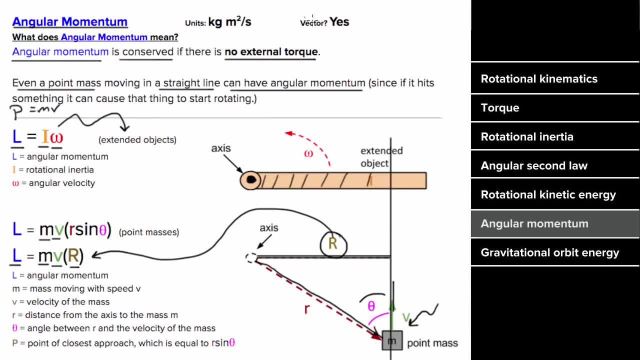 angular momentum of that point. mass Angular momentum is a vector and it's easiest to just think about the direction of angular momentum as being either counterclockwise or clockwise, depending on which way the object is rotating. And as for the units, if you multiply mass of kilograms, 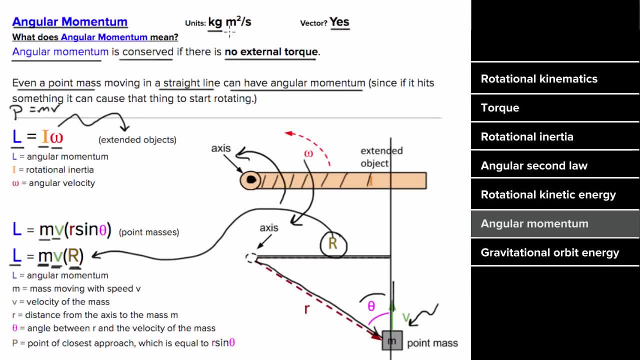 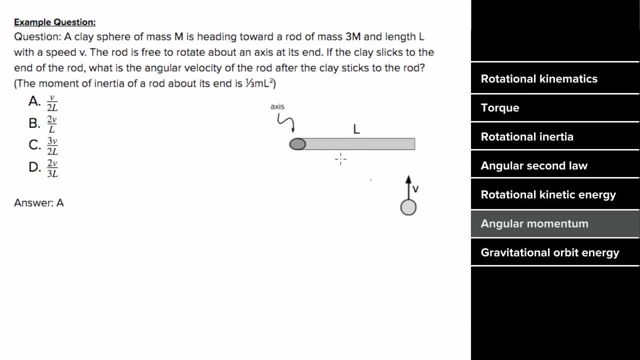 times meters per second times meters, you'd get kilogram meters squared per seconds as the units of angular momentum. So what's an example problem involving angular momentum? look like, Let's say, a clay sphere of mass m was heading toward a rod of mass 3m. 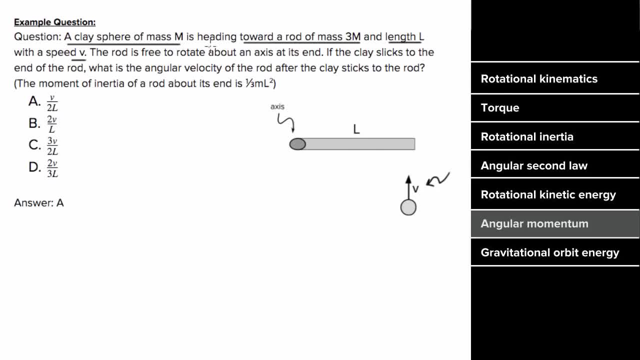 and length l. with a speed v, The rod is free to rotate about an axis around its end. If the clay sticks to the end of the rod, what would be the angular velocity of the rod? after the clay sticks to the rod And we're given? 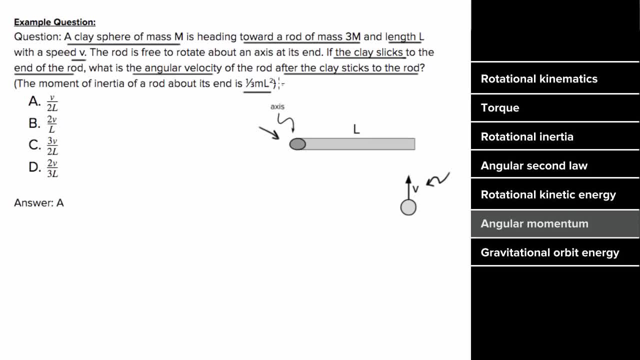 that the moment of inertia of a rod about its end is one third m l squared. Since there's going to be no net external torque on this system, the angular momentum of this system is going to be conserved, The only object in this system. 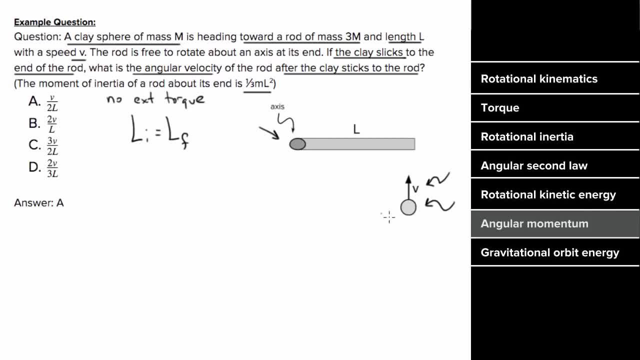 that has angular momentum initially is this clay sphere. So since this is a point mass moving in a straight line, we'll use the formula m times the velocity, times the closest it will ever get to the axis, which is l, the length of the rod That's going to. 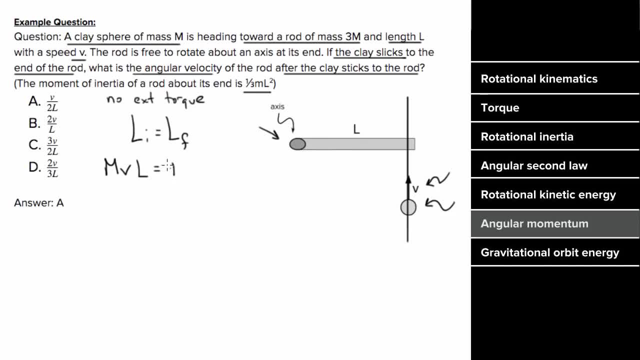 have to equal the final angular momentum, which we could write as I times omega, And this I would be the moment of inertia of both the rod and the clay that is now stuck to the end of the rod. So we'd have m v? l equals the total moment of. 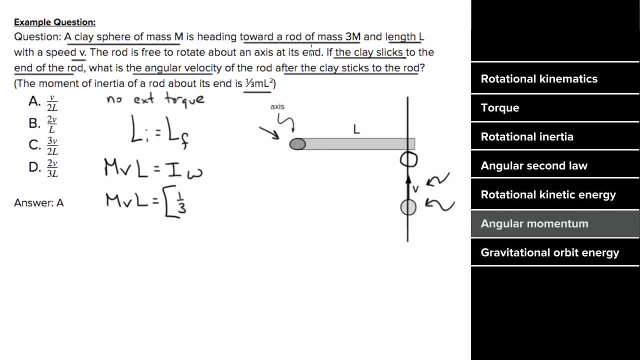 inertia. Moment of inertia of the rod is one third mass of the rod, which is 3m times the length of the rod squared, plus the moment of inertia of this piece of clay stuck to the end of the rod, rotating in a circle, is going. 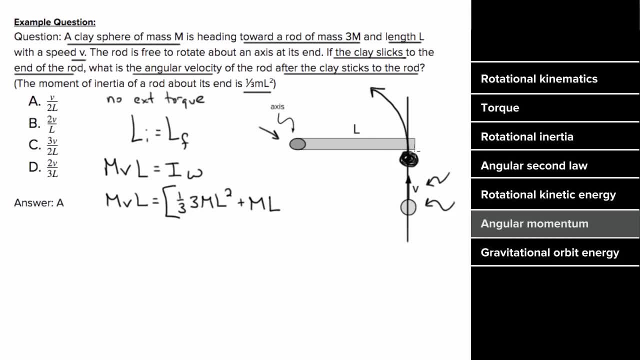 to be the mass of the clay times the radius of the circle that clay traces out, which is the length of the rod. In other words, we're using the formula for the moment of inertia of a point mass whose entire mass is rotating at the same radius from the center. 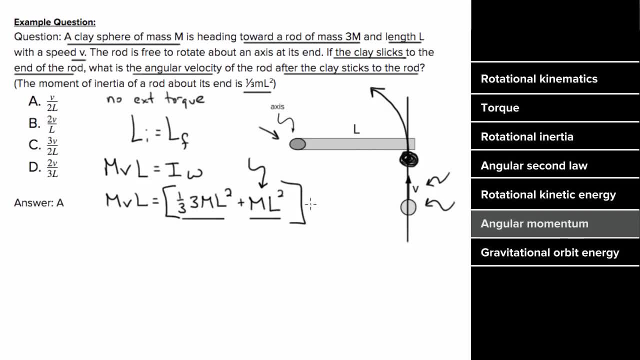 And we add that to the moment of inertia of the rod itself. We multiply by omega, The term in brackets comes out to be 2m l squared. We can cancel the m's, we can cancel one of the l's and we get. 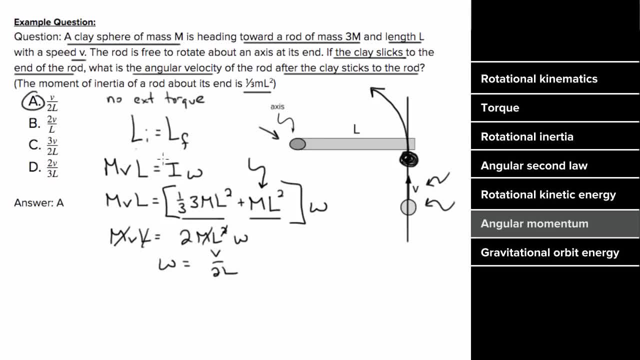 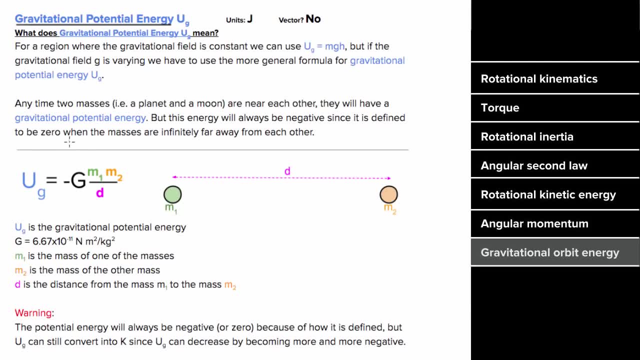 that omega is going to equal v over 2l. The last topic I want to talk about is the more general formula for the gravitational potential energy. Why do we need a more general formula? Well, if you're in a region where the gravitational field little. 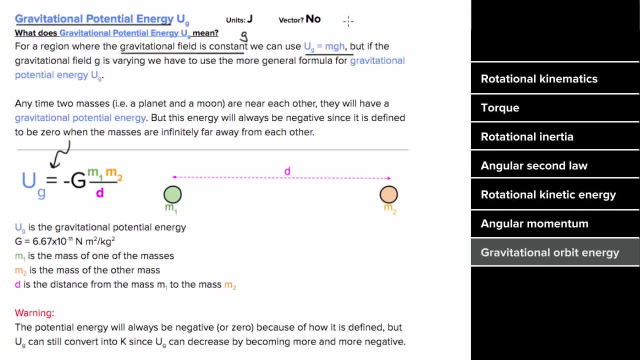 g is constant, then you could just use our familiar formula m, g, h to find the gravitational potential energy. But if you're in a region where the gravitational field is varying, then you have to use this more general formula which states that the gravitational potential 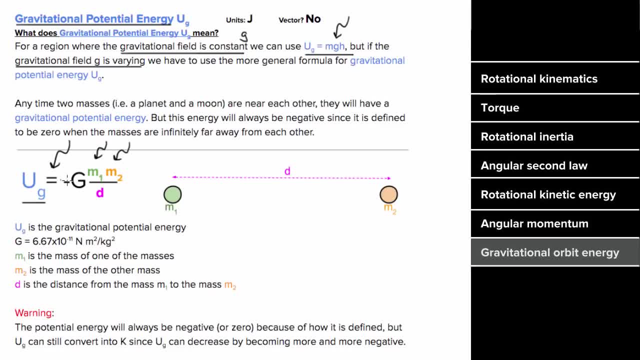 energy between two masses, m1 and m2, is going to equal negative of the gravitational constant. big G times the product of the two masses divided by the center to center distance between the two masses. Note this is center to center, not surface. 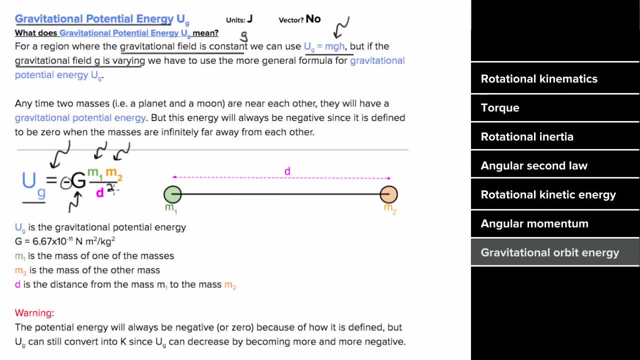 to surface and it's not squared like it is in the force formula. This one's just the distance. Gravitational potential energy is not a vector, but because of this negative sign the gravitational potential energy is always going to be negative or zero. 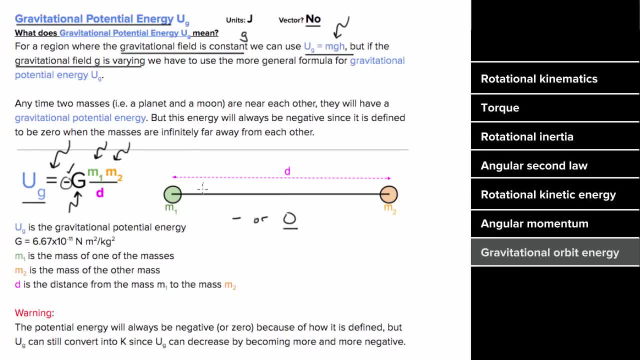 It'll only be zero when these spheres become infinitely far apart, because then you'd divide by infinity and one over infinity would be zero. Otherwise it's always negative. But even though this gravitational potential energy is negative, this energy could still get converted into kinetic energy. it's just. 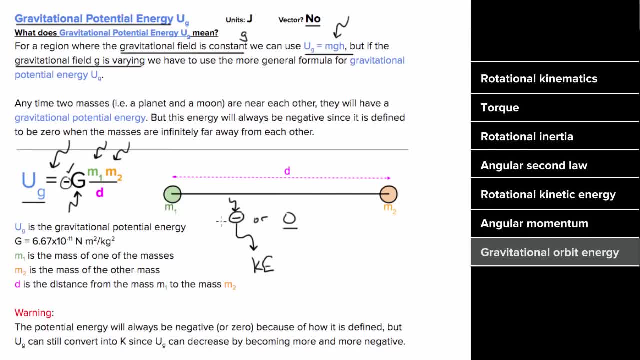 that in order for this gravitational potential energy to decrease, it would have to become even more negative to convert that energy into kinetic energy. I'm bringing up this topic in this section because oftentimes, when planets are orbiting each other in circular orbits, you have to use this formula to determine. 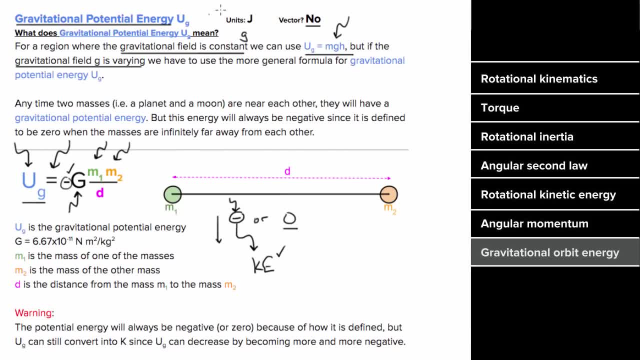 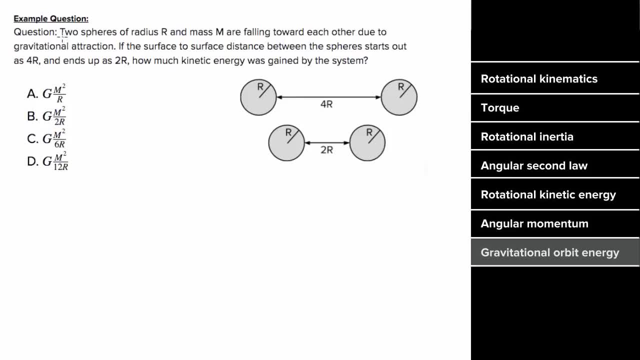 the gravitational potential energy between them And since it's an energy, the units are joules. So what's an example problem involving this more general formula for the gravitational potential energy? look like, Let's say, two spheres of radius r and mass m are falling toward each other. 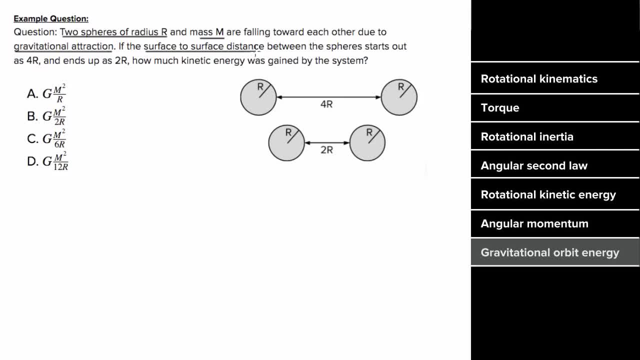 due to their gravitational attraction. If the surface to surface distance between them starts off as 4r and ends up as 2r, how much kinetic energy would be gained by this system? We'll include both masses in our system, and that would mean 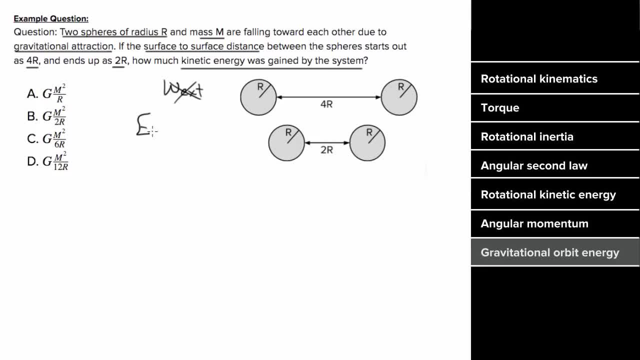 that there's going to be no external work done. so the energy of this system is going to be conserved. The system is going to start off with gravitational potential energy negative big G, both masses multiplied together, which is m squared divided by the distance they start off. 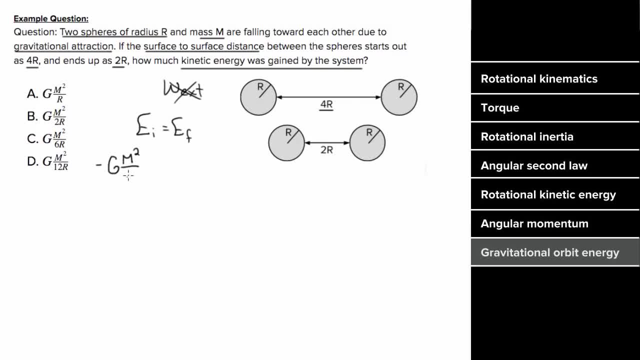 from each other, which is not 4r, it's the center to center distance, which is going to be 6r. We'll assume they start from rest, so there will be no kinetic energy to start with. This is going to equal the final gravitational. 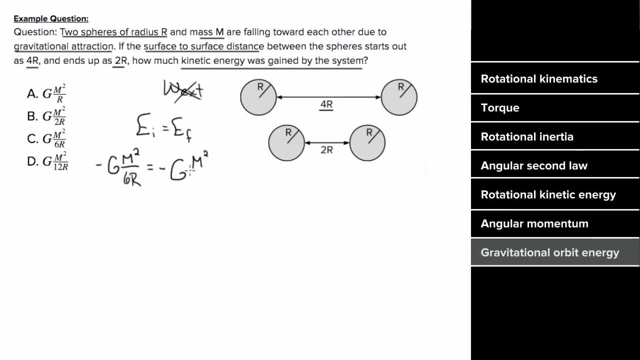 potential energy. negative big G. both masses multiplied m squared, divided by the distance they end up, which is not 2r, it's the center to center distance, so that's 4r plus however much potential energy was converted into kinetic energy. 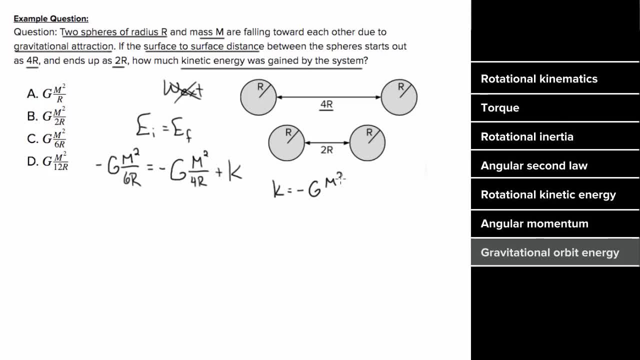 If we solve this for kinetic energy, we're going to get negative big G m squared over 6r plus big G m squared over 4r. 1 fourth minus 1 sixth is going to be 1 twelfth. 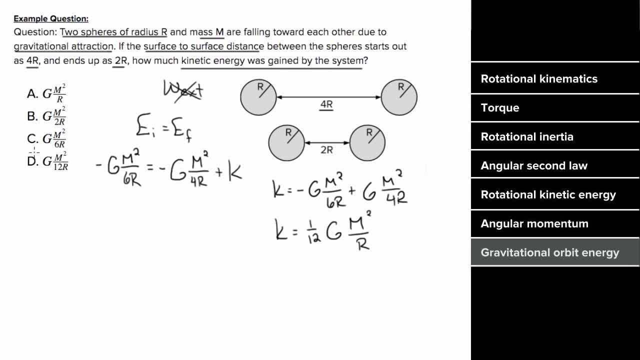 so the amount of potential energy that was converted into kinetic energy would have been big: G m squared over 12r.